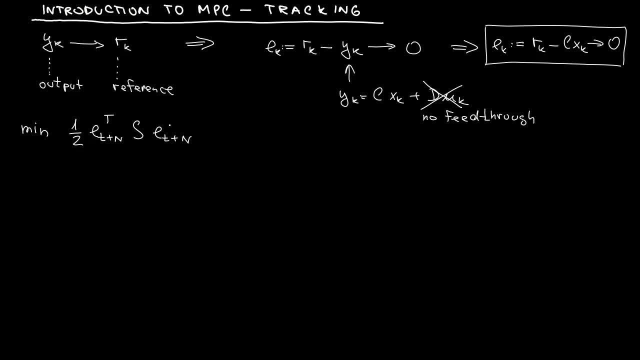 Starting with the term penalizing the situation at the final time. Of course, this will always have to be done at every sampling period. So, just replacing the state with the regulation error in the optimization criterion And that, perhaps, that this will be it. 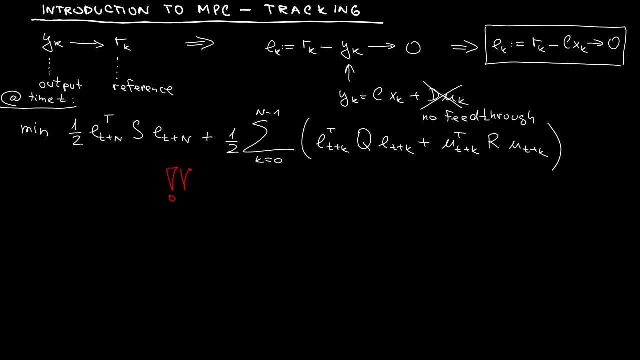 Unfortunately, this is not the case. The situation is not as simple as that. Why? Well, it's simply because that Your desire is to see in a steady state the regulation error equal to zero, But at the same moment, you can't have the control equal to zero in general tracking situation. 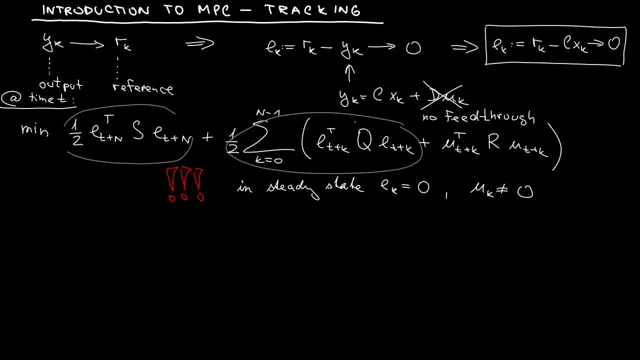 But then in optimization, if the regulation error is equal to zero, these terms must vanish, whereas this guy will not vanish. But now the optimization is not aware of your problem. so what it will do is that it will try to bring the term corresponding to control close to zero. 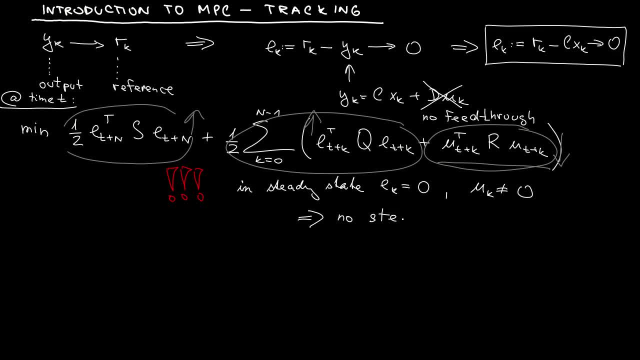 And the terms corresponding to the regulation error it will drive away from zero. That means with this control scheme you will not be able to have zero error at steady state. What's the solution? The solution is to use the increment of control signal instead of the control signal itself in your model. 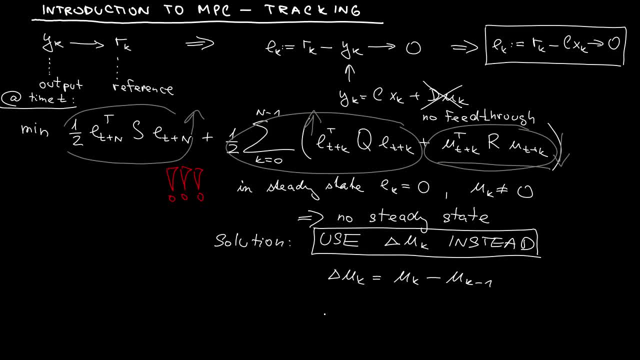 The control increment is defined as uk-1.. That means the value of the control signal minus the value of the control signal. That's the value of the control signal in the previous time step. Now, if I reformulate this, I can express my control signal at time k as the control signal at the previous time step plus the increment. 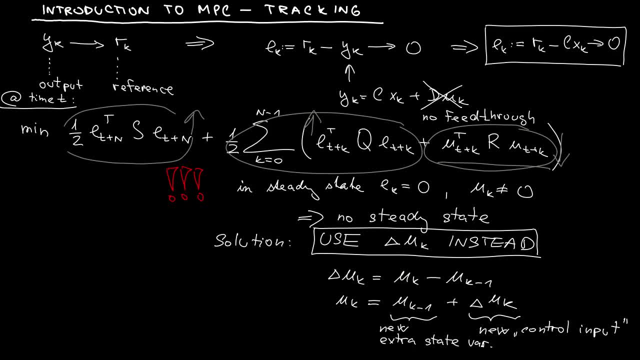 Now the increment is regarded as the new control signal, whereas the value of the control in the previous time step is our new state variable. So let's now incorporate this new state variable in our state-space model. We will have to augment it. 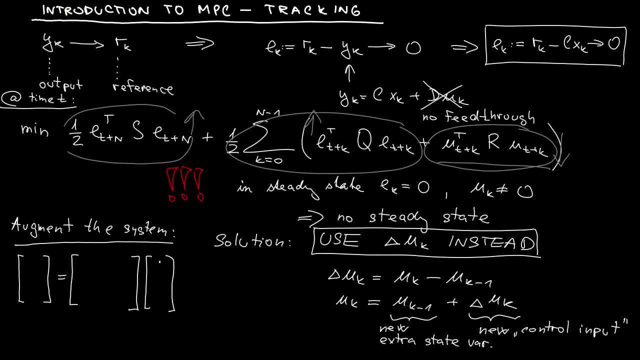 We will have to augment the original state vector x. The new vector will be augmented with the state vector x, with the upper index u, which will stand for the value of control in the previous time step, And similarly, instead of the original input u, I will have just delta u as my new control input. 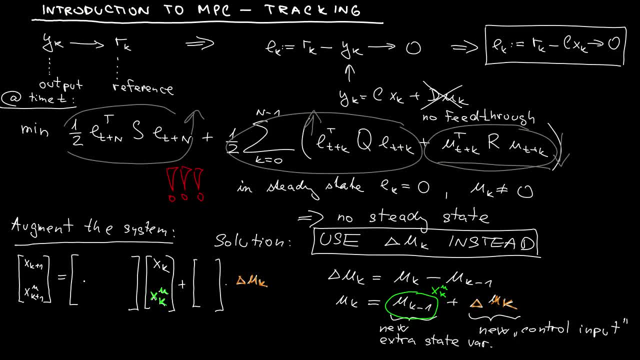 All right, Filling in the matrices here is pretty straightforward, as you can verify by yourself, And now I will label the new augmented state vector as x- tilde, And this will be new state matrix A- tilde and B- tilde. 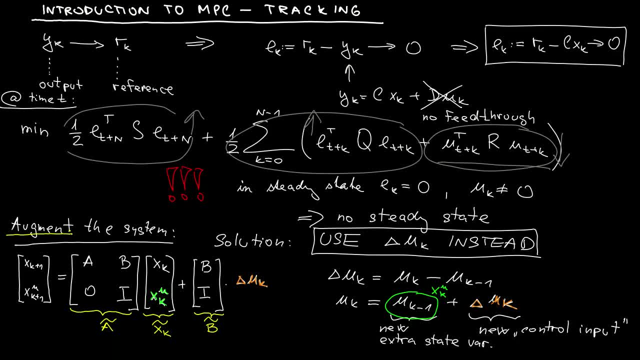 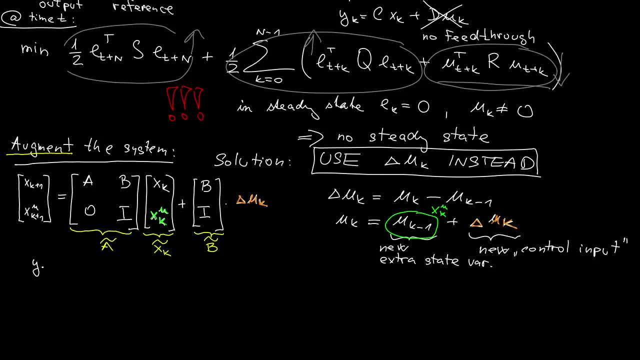 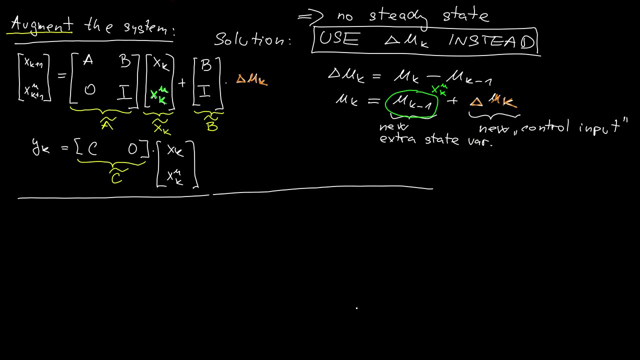 So remember that whatever has tilde here relates to the augmented system. All right, Now with this new state vector, I will express the output in the following way: Again, the C tilde matrix. And now, with this new state-space model, I will write down the optimization cost as again the term corresponding to the regulation. error in the final time. 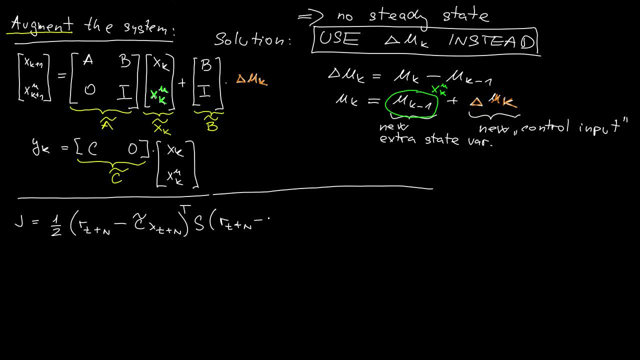 And plus the so-called running costs. That means costs between the initial and final time Now plus the term corresponding to the increment of u. It can't fit here, so I'll move it on the new line. Oops, I forgot to add the delta term. 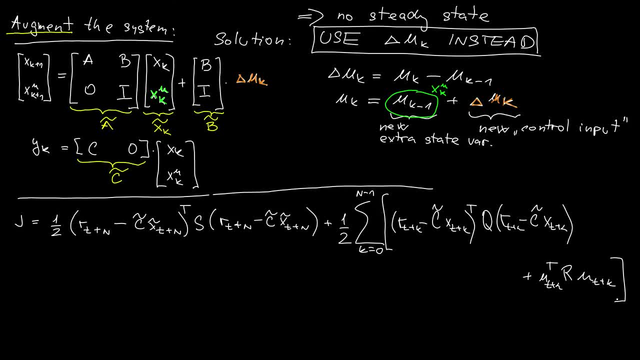 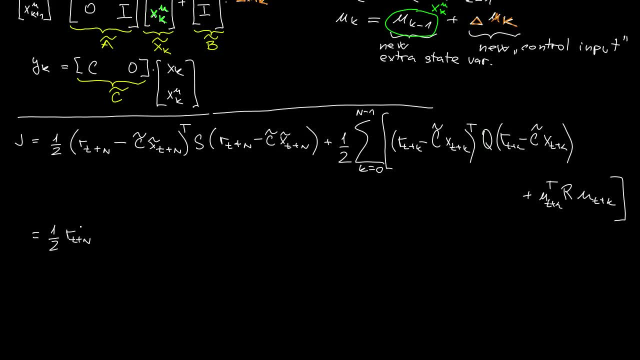 I will correct it later. So now let's factor out the terms here. Now you don't have to be worried, Your loudspeaker is still functional. It's just that. there's not much I can do. There's not much I can add here. 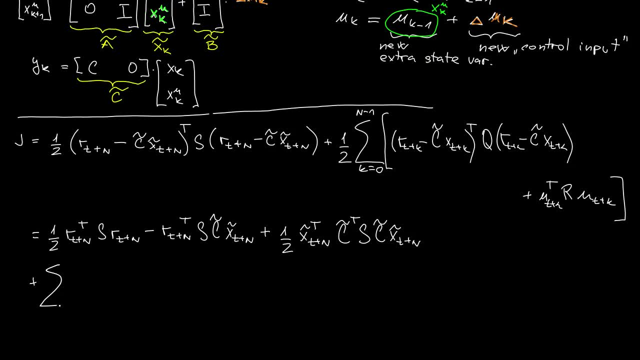 And finally the running cost Time for a little snack. Yeah, the term that is quadratic in X. And finally the term that is quadratic in the new control Here. I correctly have deltas here, So that's it. I will also correct it up there. 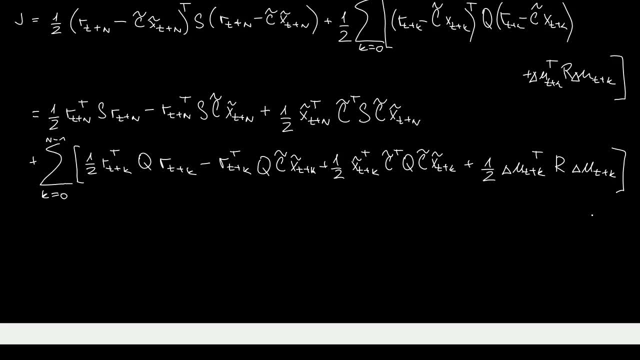 All right. So the usual procedure then was to cancel the constant terms, The terms that only contain the references here. Of course, it then gives a new cost function, which I should have labeled differently. But well, if you tolerate this abuse of notation, I will keep labeling this cost function, just as J. 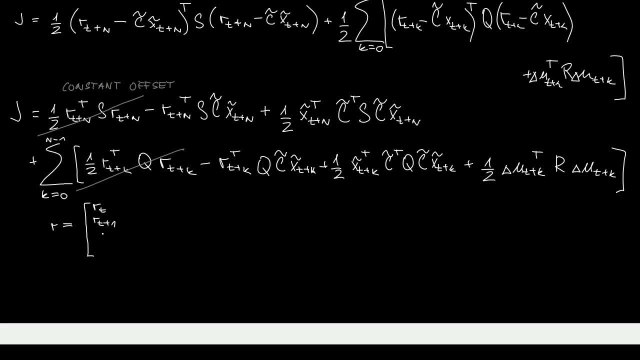 And now I will reformulate this cost function using those long stacked vectors which contain the values of the corresponding variables over all time instances, over the whole interval. So R now stands for the long vector, R with references X. tilde is a long vector with the augmented states. 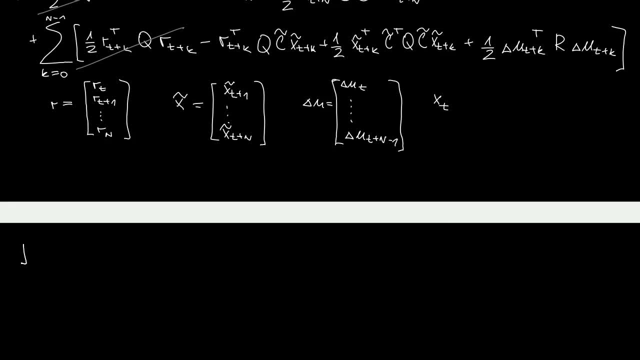 And similarly for delta use And Xt is, of course, the value of the state at the beginning, The value of the state at the beginning of our horizon. Now I can rewrite the cost function in this format of long vectors as this: 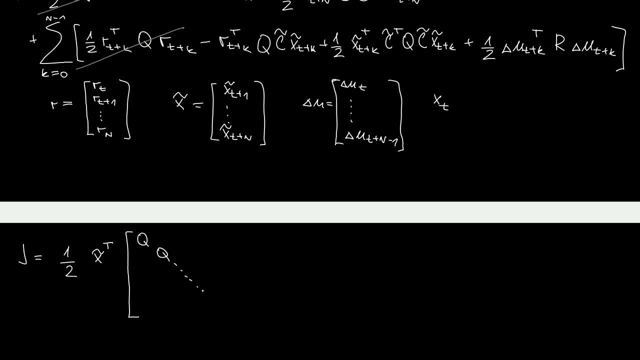 So here I will have the term that corresponds to squared X tilde, Then I will have a term that is linear in X tilde And finally the term that is quadratic in controls, or actually in the increments of the control signal. 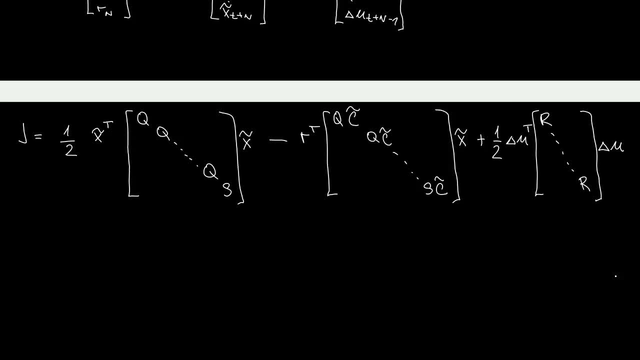 Now, this is actually the cost function. That means I will want to minimize this subject to the following constraints: And now, the format of the constraints is pretty much identical to what you have seen in the previous videos. It's just that here, instead of X, we have X: tilde. 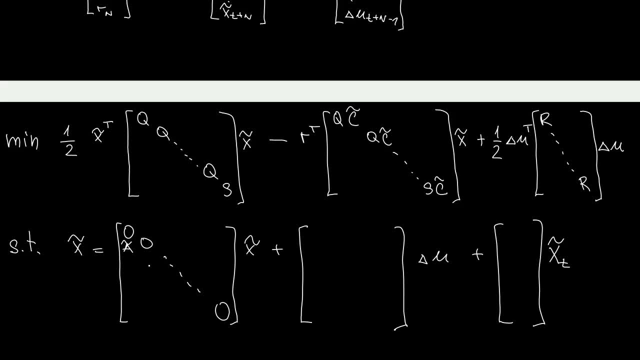 Instead of U we have delta U And so on. But other than that, the structure is identical. So for later convenience, let's label these matrices with their own names. Perhaps I will use double bar to indicate that the matrices belong to the tracking problem. 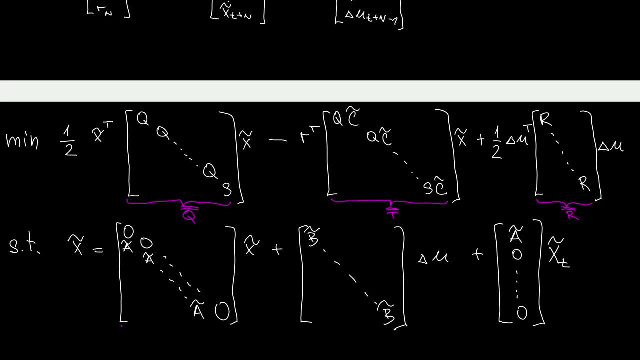 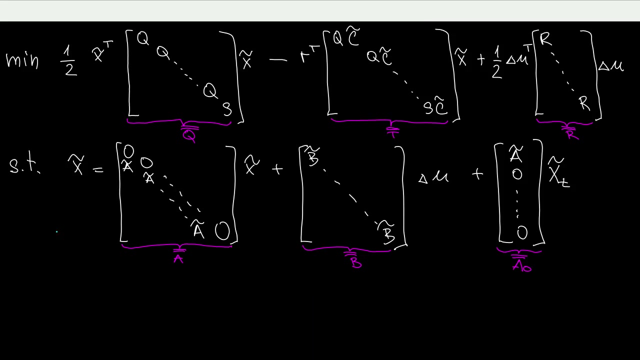 So Q double bar, T double bar, R double bar, A double bar, B double bar, And this could be perhaps, say, A double bar zero. And in fact that's it. We are now almost ready to call a solver for quadratic programming. 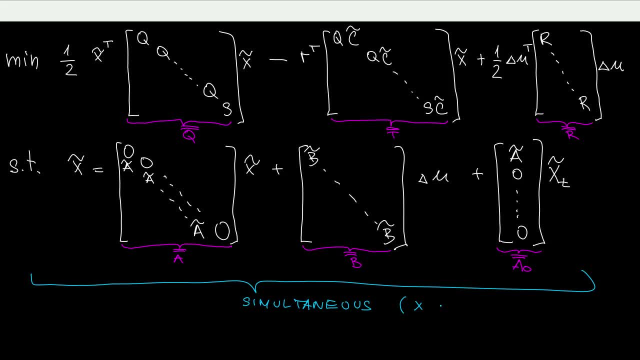 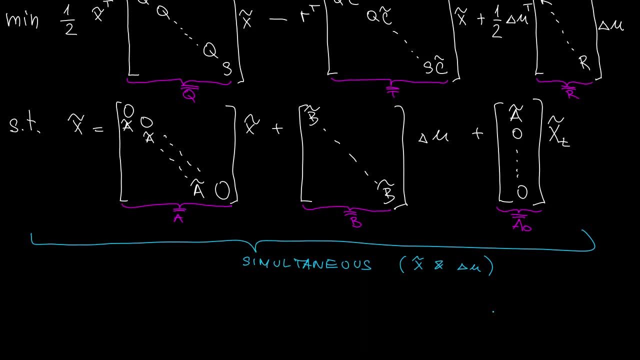 We have formulated our optimal control problem in the so-called simultaneous format. Simultaneous because we have both X tilde and delta U. However, you know that it's actually a pretty good idea to eliminate the state variables using the state equations and express the whole optimization purely as an optimization over delta U's. 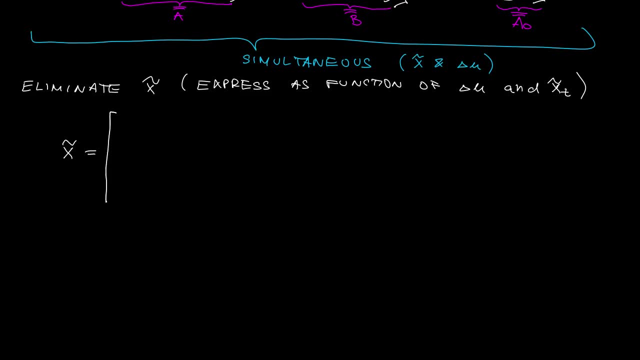 All right, so now let's go for it Again. the relationship that we will use to eliminate the X tilde is pretty much identical in structure to the relation that we have. It's the same thing that you have seen in the previous videos. 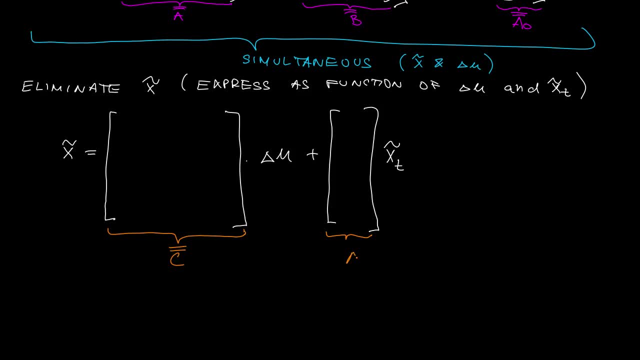 It's only that now I will have double bar matrices, C double bar and A double hat, The matrices that relate X double bar, X tilde and the increment in U and the augmented state at the beginning of the horizon. All right, so now I will take this expression for X tilde. 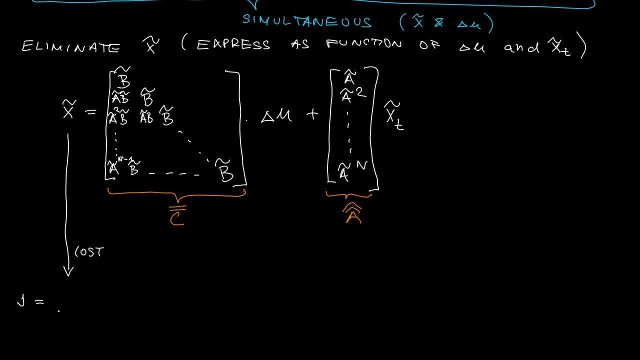 and substitute it into the cost function. So instead of X tilde I will have the following term here: Q double bar and again the term corresponding to to X tilde, And then I will have the term that corresponds to to the increment in control. 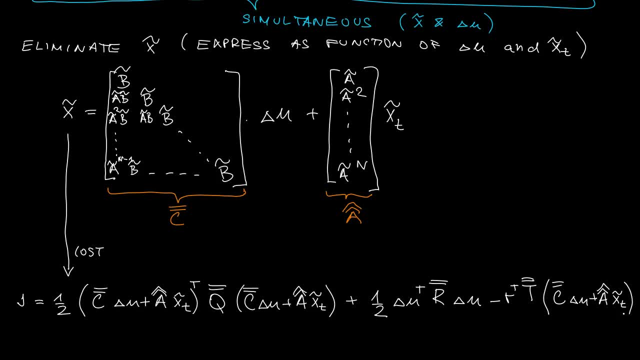 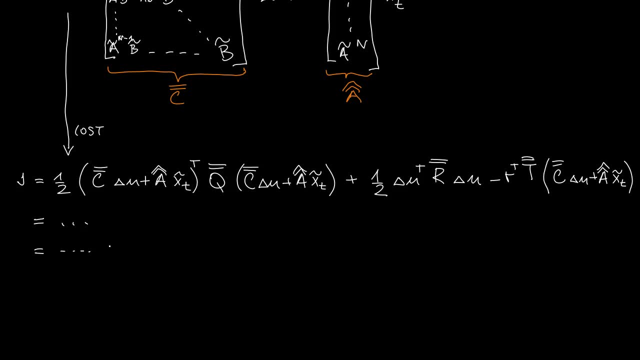 And finally the cross product. here And now, this will really be just a matter of one or two lines Of straightforward but tedious derivation. You will also- you may also want to ignore the constant terms, because they add nothing. So, with the common abuse of notation, 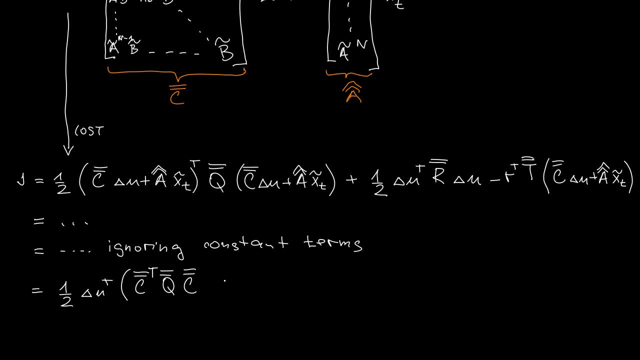 I will just keep using the same letter G for the cost function, And let me now show you the outcome. So what we will arrive at is the expression for the cost function, which contains the term that is quadratic in delta U and the term that is square. 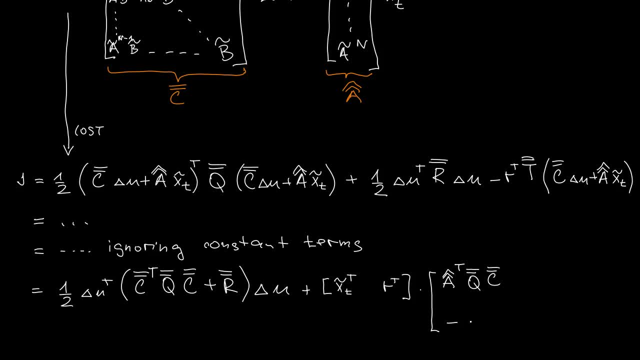 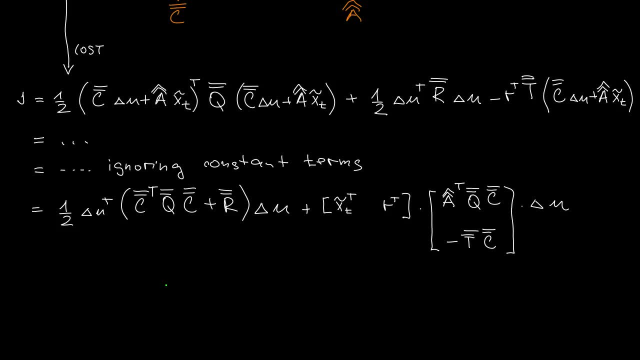 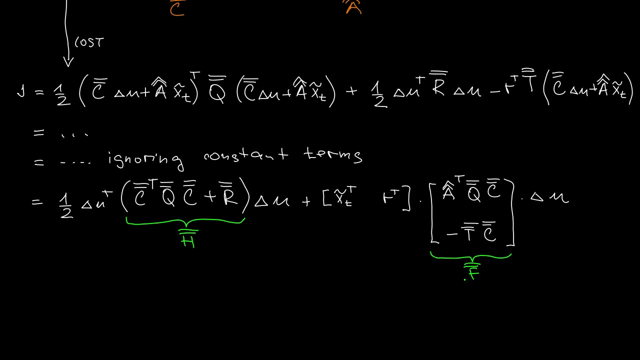 It is linear in delta U, And the structure of this expression is already very much familiar. right, By labeling the two matrices as H double bar and F double bar, I can now write the cost function in this compact form. So the quadratic term and now the linear term. 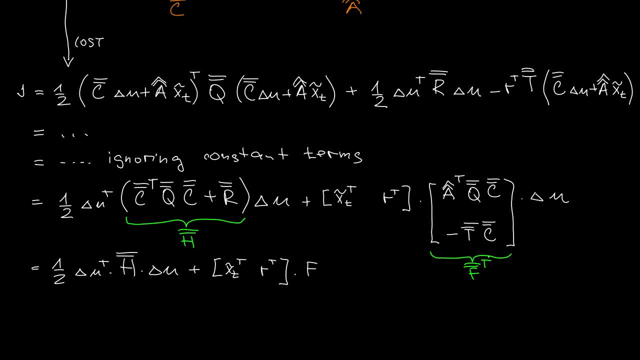 which is also parameterized by the value of the augmented state. Yeah, now F matrix should actually be transposed, And I forgot to include double bar up there. Anyway, by differentiating this cost function with respect to delta U, this is what I obtain. 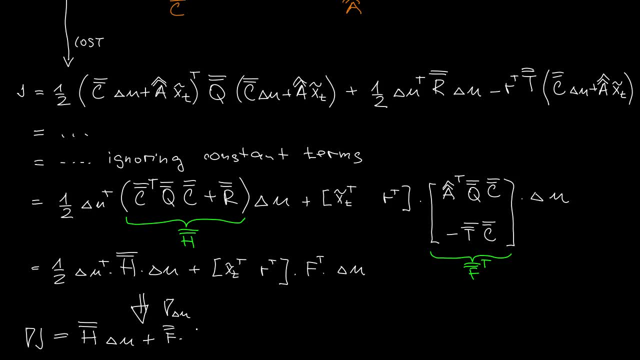 That means a function that is linear- linear in delta U- And this should be equal to zero. So in absence of constraints, I will find my optimal sequence of delta U's by solving a set of linear equations. If there are some constraints- inequality type constraints- 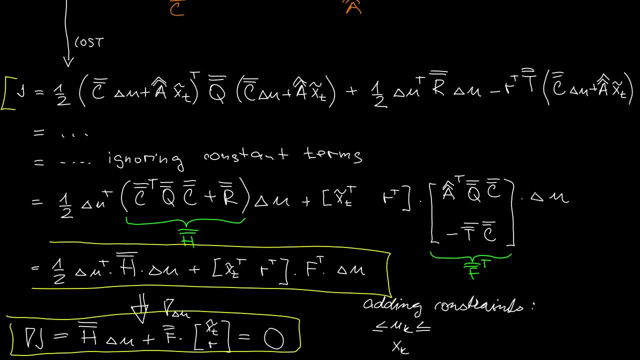 for instance bounds on the control signal, which is now part of the augmented state vector, and bounds on the state variables themselves. Well, we will then use the following expression: relation between X, tilde and delta U's And simply formulate standard QP problem. 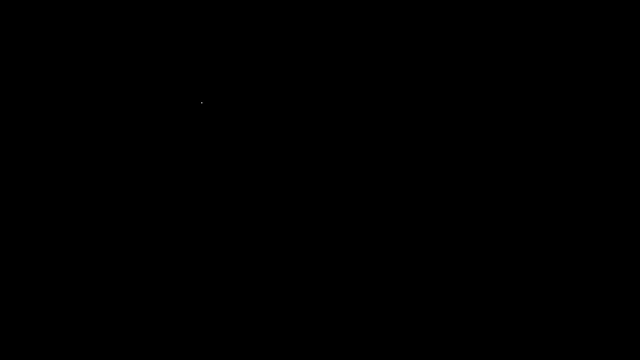 with linear constraints. Now, one issue, practical one, that I would like to discuss is the capability of an MPC tracker to behave in an anticipatory way, should provide so-called preview capability. So let me consider the following scenario: I find myself, or the controller finds itself at time t. 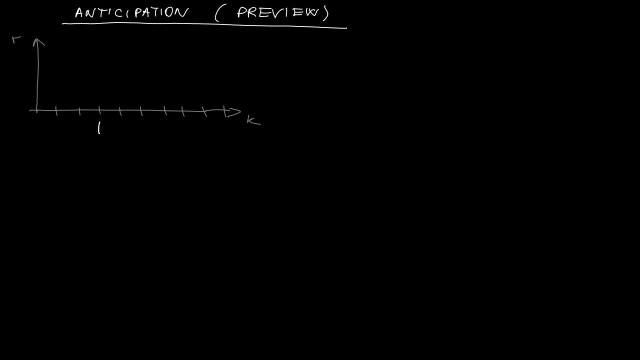 discrete time t. So this is what we will regard as the presence, This is the current moment, And then the considered shape of reference signal looks like this: Now, although in MPC we are doing optimization, over some window, some horizon, the value of the reference signal. 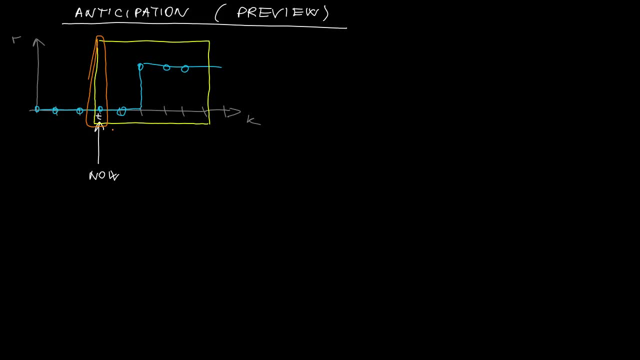 is only known at the current moment, So we do not know that two steps later there will be a step. Therefore, the resulting behavior of this system, the evolution of the output, will look like this: It will only start responding those two steps later.